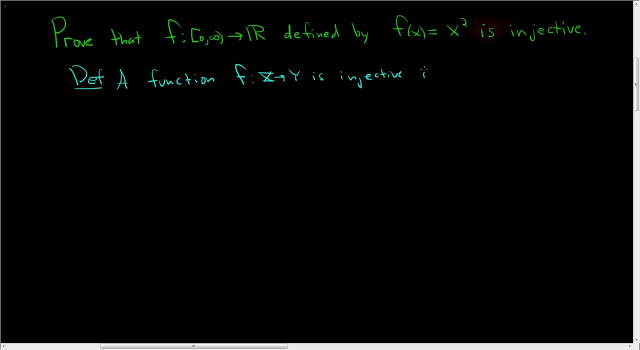 if for all ab in the domain of our function, whenever we have equal outputs, so f of a is equal to f of b, then the inputs must also be the same. a is equal to b. So equal outputs, equal outputs. So f of a is equal to f of b. 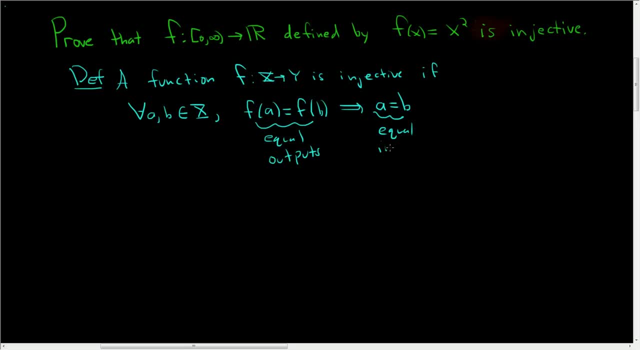 So f of a is equal to f of b, give rise to equal inputs. There's lots of ways to think about an injective function, lots of really, really cool ways, but in this video I just want to focus on the proof. 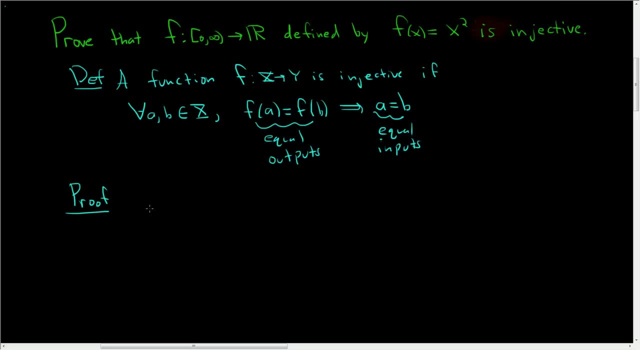 So proof All right. so to use this definition, we have to start by supposing that we have F of A equal to F of B for some arbitrary A B in the domain of F. So in this case, this is our big X, our capital X. So A B will live inside the 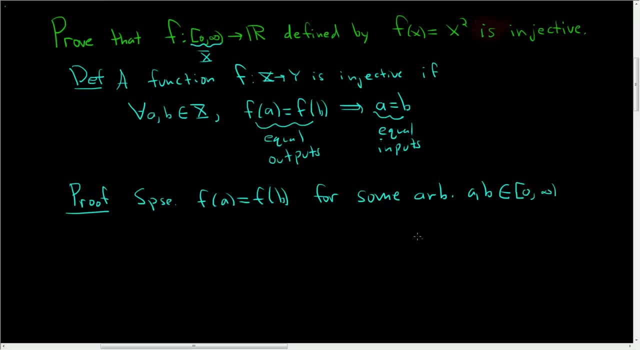 interval from zero to infinity, which includes zero. Okay, now we just have to show that A is equal to B. So we started by assuming that F of A is equal to F of B. for some arbitrary A, B in the domain of F. 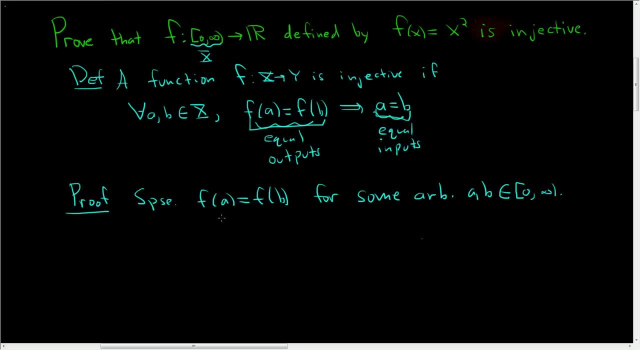 And we have to prove that A is equal to B. Well, F of A? well, what is that? Well, F of X is X squared, So F of A is A squared, And this is equal to F of B, which is just B squared. 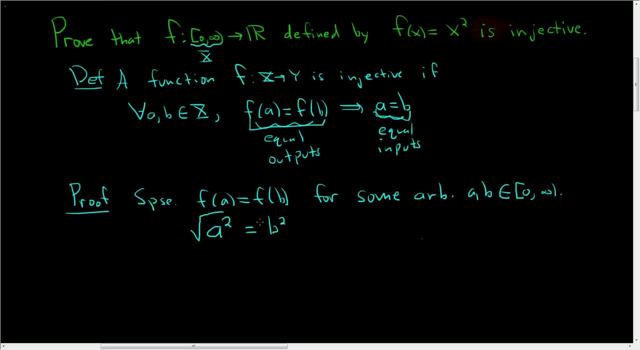 So the natural thing to do next is to take the square root of both sides. So when we do that we get the absolute value of A equals the absolute value of B. But you'll notice that A and B are both equal. They're both greater than or equal to zero. 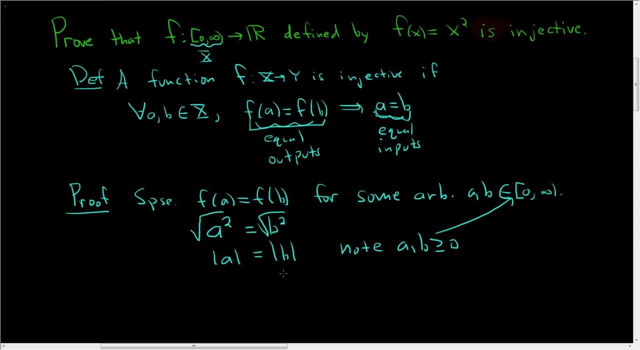 Why? Because they're in this set here. So the absolute value of A is just A And the absolute value of B is just B. Since A and B were arbitrary, this holds for all A- B in our domain. Thus F is injective.